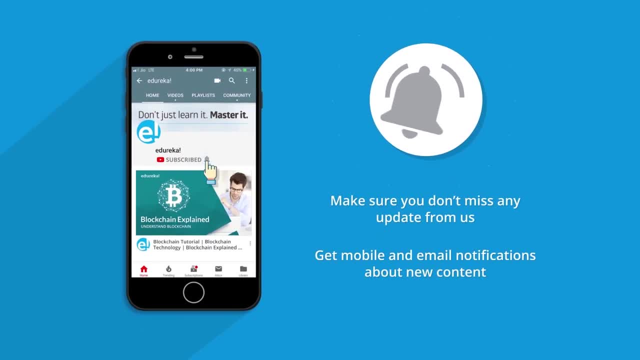 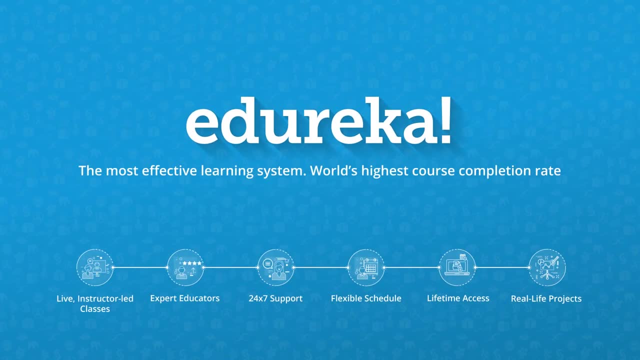 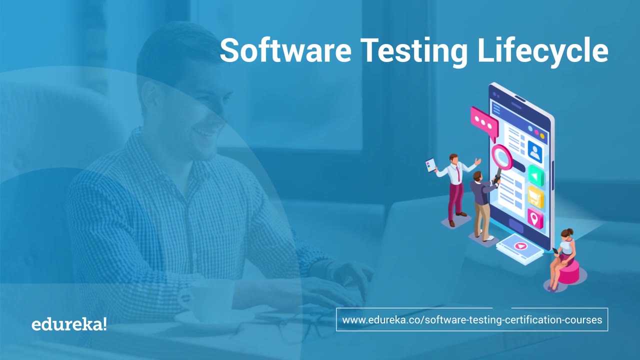 Today's world of technology is completely dominated by machines, and their behavior is controlled by the software powering it. Now, will the machines behave exactly as we want them to, every time and everywhere? The answer to these questions lie in software testing. Hi everyone, this is Shainthini from Edureka, and today we are going to have a look at the 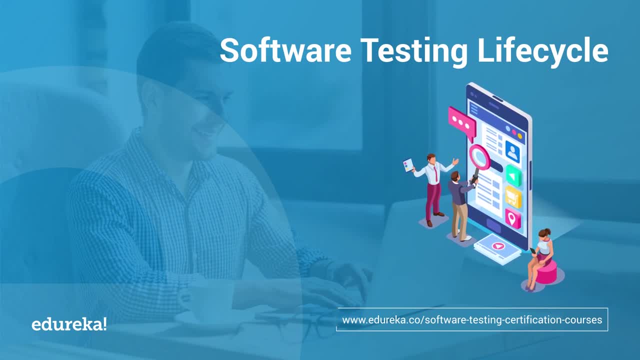 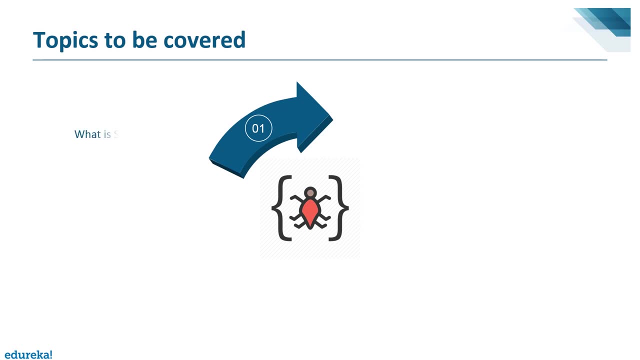 different stages of software testing, known as the software testing life cycle. So let's have a look at today's agenda first. So we shall start with a brief introduction to software testing and then we will see why software testing is important. Next up, we will see who does the software testing. 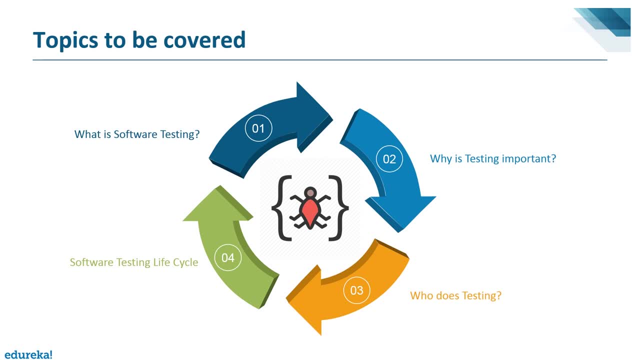 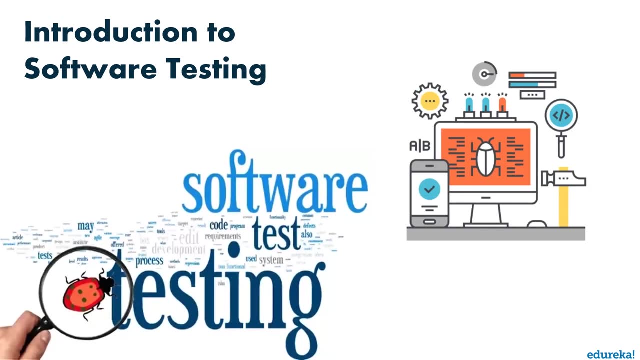 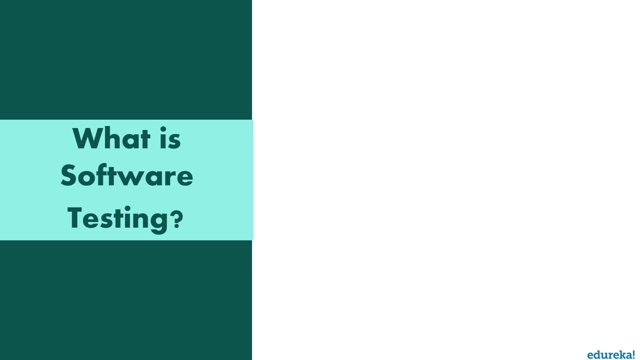 and then we will move on to the six different phases involved in software testing life cycle. So let's get started Now. the last decade has seen an overwhelming evolution of the software testing industry, giving way to greener pastures. Now it is important to ensure. 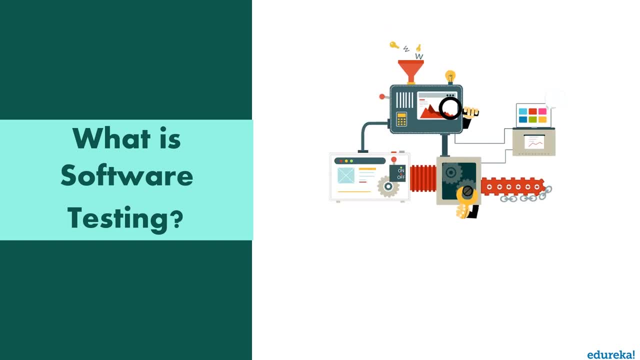 an effective performance of software application, and software testing is required to ensure that the application runs without any failures. Now, software testing is a process of evaluating the functionality of a software application to find any software bugs. It basically checks whether the developed software met the specified requirements and identifies any. 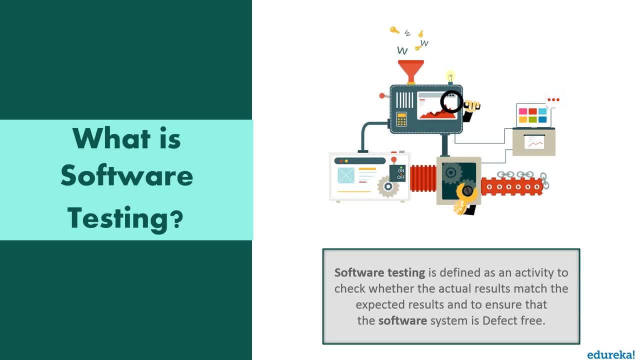 defect in the software in order to produce a quality product. It is also stated as the process of verifying and validating a software product. It basically checks whether the software product meets the business and technical requirements that guided its design and development. It also works as part of the requirement. It can also be implemented with the 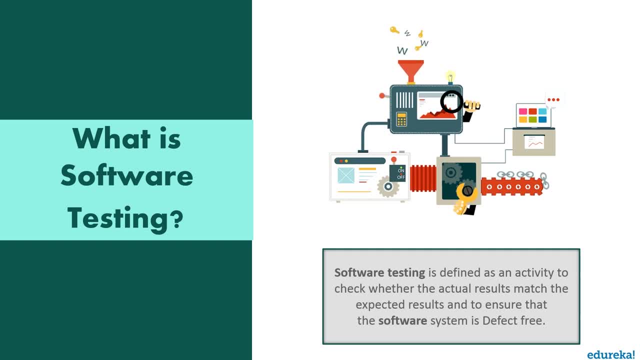 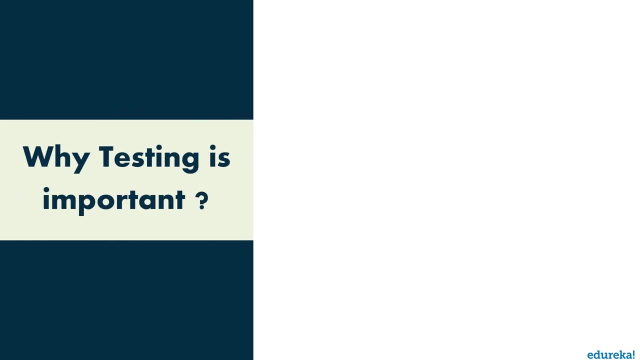 same characteristics. Now, the software testing group is a service provider, So the software testers provide valuable information and insights into the state of the system. Now this information contributes towards reducing the ambiguity about the system, For example, when deciding whether to 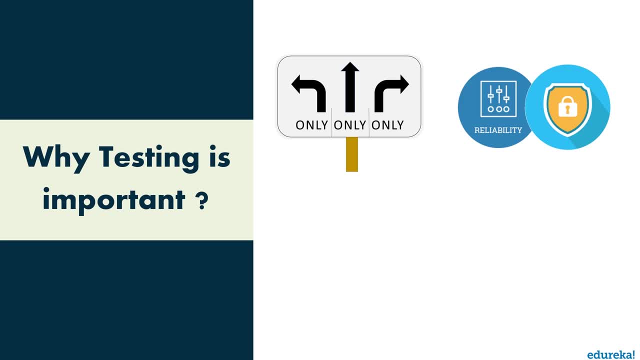 release a product, the decision makers would need to know the state of the product, including aspects such as the conformance of the product to requirements, the usability of the product and the product, any known risks, the product's compliance to any applicable regulations, etc. Software. 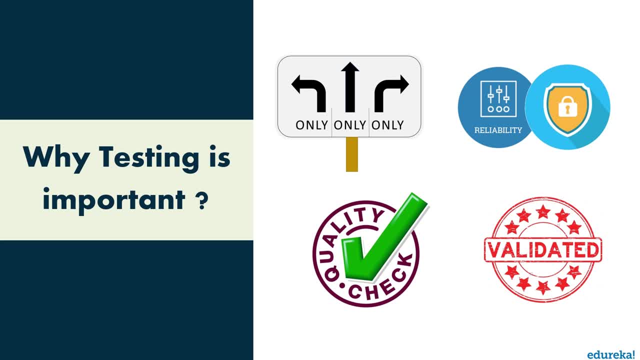 testing enables making objective assessments regarding the degree of conformance of the system to stated requirements and specifications. So testing verifies that the system meets the different requirements, including the functional performance, reliability, security, usability and so on. And this verification is done to ensure that we are building the system right Now in 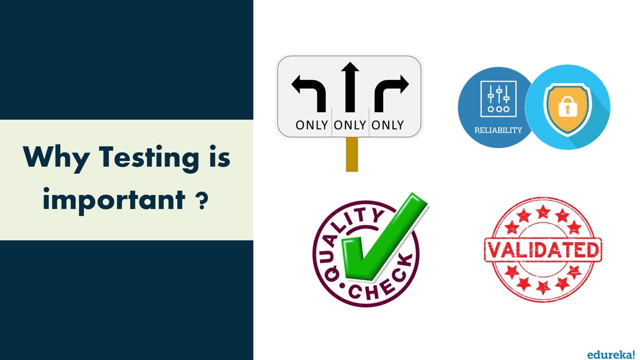 addition, testing validates that the system being developed is what the user actually needs. In essence, validation is performed to ensure that we are building the right system And, apart from helping make the decisions, the information from software testing helps with risk management. Software testing contributes to improving the quality of the product. Not just that software. 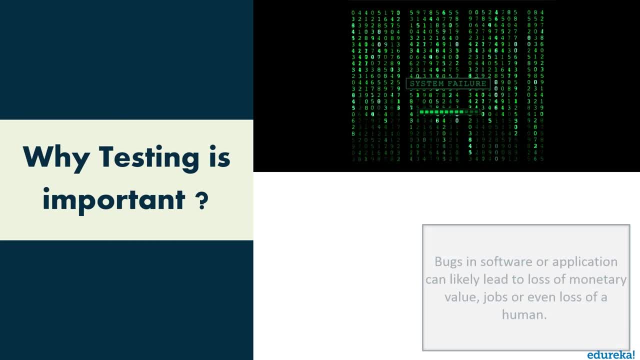 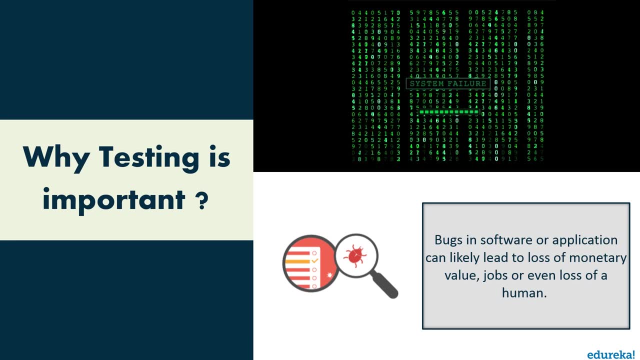 testing also points out the defects and errors that were made during the development phases. It looks for any mistake errors that were made by the programmer during the implementation phase of the software. It ensures that the customer finds the organization reliable and their satisfaction in the application. 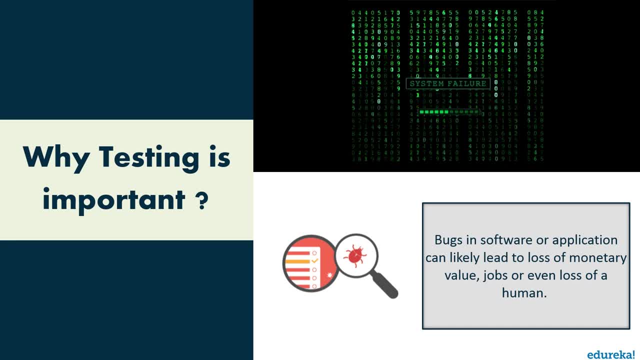 is maintained. Sometimes contracts include monetary penalties with respect to the timeline and quality of the product, and software testing prevents the monetary losses. It also ensures quality of the product. So quality product delivered to the customers helps in gaining their confidence. It makes sure that the customer is satisfied with the quality of the product. 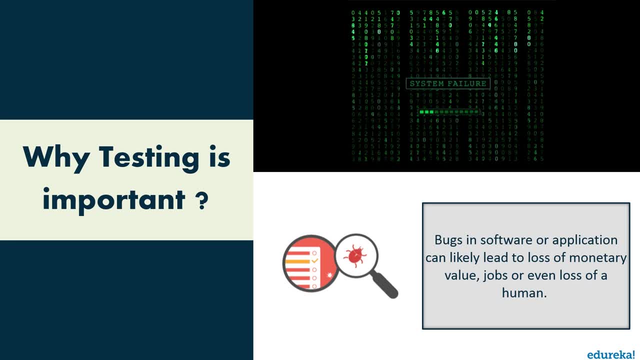 So quality product delivered to the customers helps in gaining their confidence. It makes sure that the software application requires lower maintenance cost and results into more accurate, consistent and reliable results. Now the users are not inclined to use software that has bugs They may. 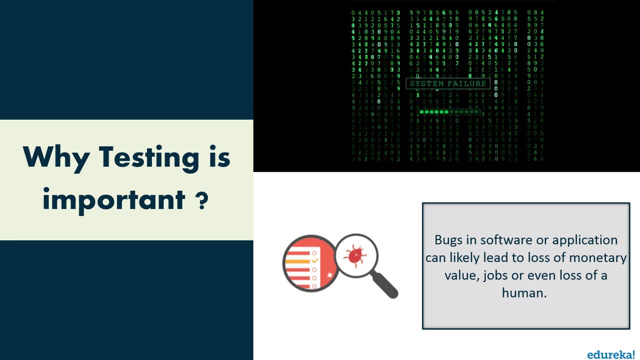 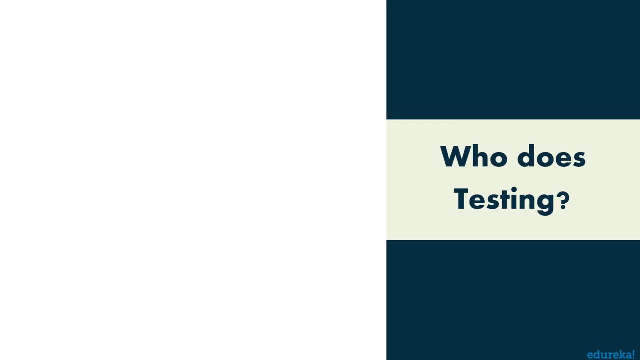 not adopt the software if they're not happy with the stability of the application. So testing is very important for the product to stay in business. So now let's have a look at who does this software testing. So for that we have the software testers, project lead or managers. Then we have 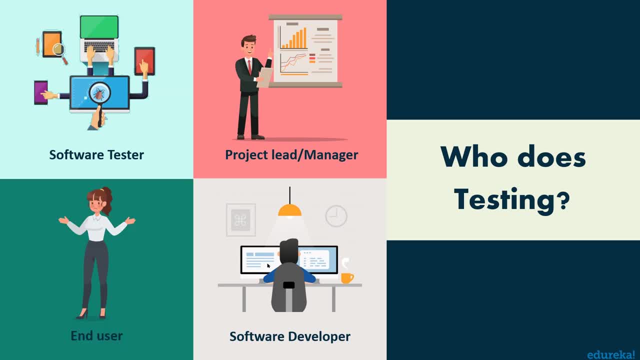 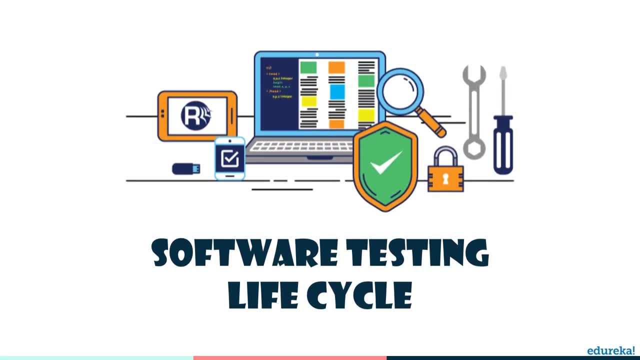 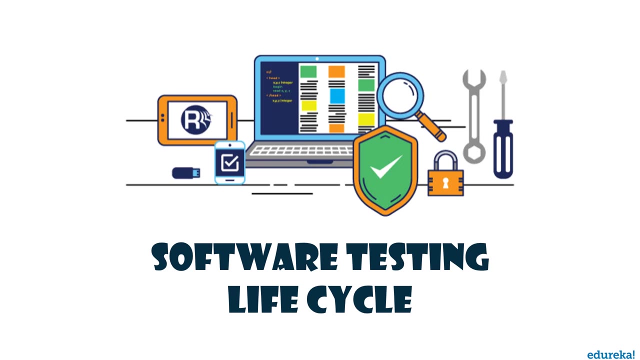 software developers. And also, finally, we have the end users that perform the software testing before any software application is developed. So now that you know what is software testing and who performs this testing, let's move on and have a look at the software testing life cycle. 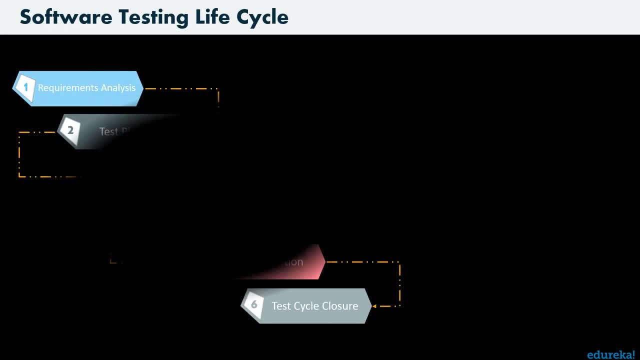 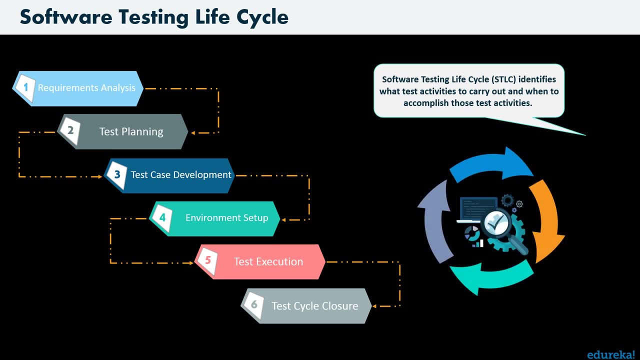 So the software testing life cycle, or the STLC, defines a series of activities conducted to perform the software testing Now. it defines what test activities to carry out and when to accomplish those test activities. So in software testing life cycle process each activity is carried out in a planned and systematic way and each phase has different. 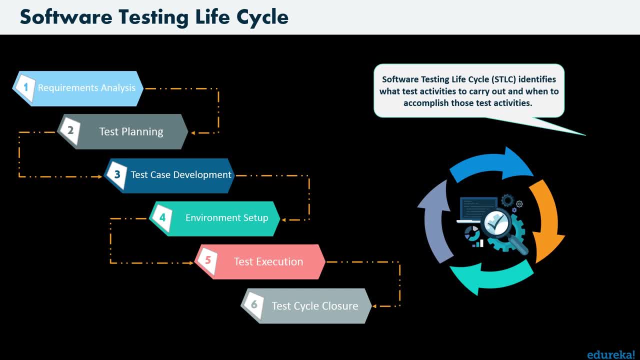 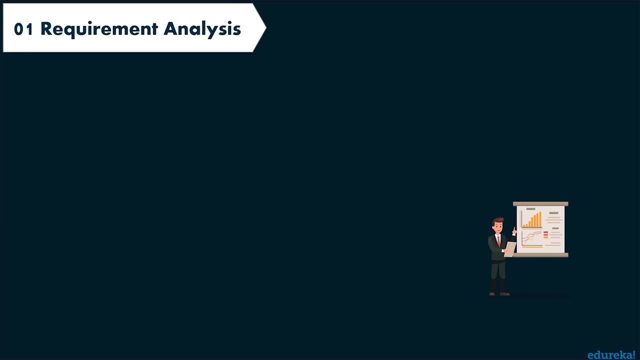 goals and deliverables. Now, the different phases of software testing life cycles are the requirement analysis, test planning, test case development, environment setup, test execution and, finally, the test cycle closure. So let's start with the first phase of that is the requirement analysis. 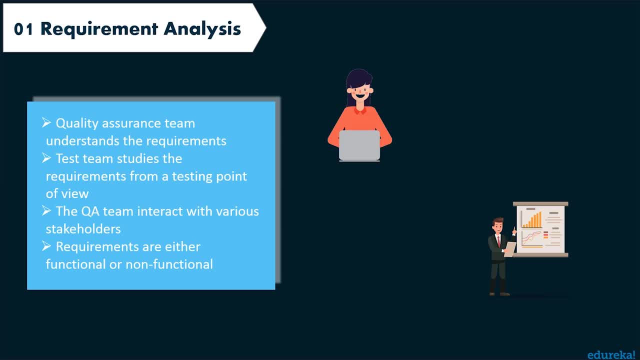 Now the requirement analysis is the first step involved in software testing lifecycle And in this step, quality assurance team understands the requirement in terms of what we will be testing and figure out the testable requirements. Now, during this phase, test team studies the requirements. 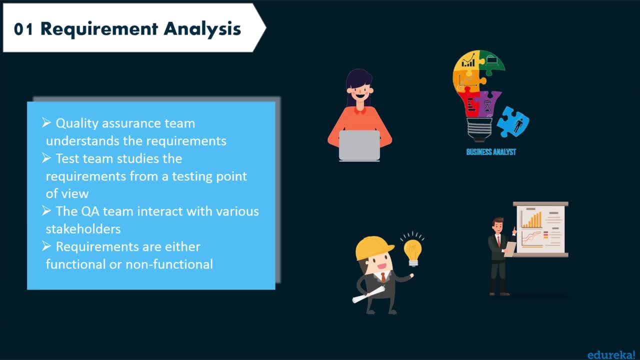 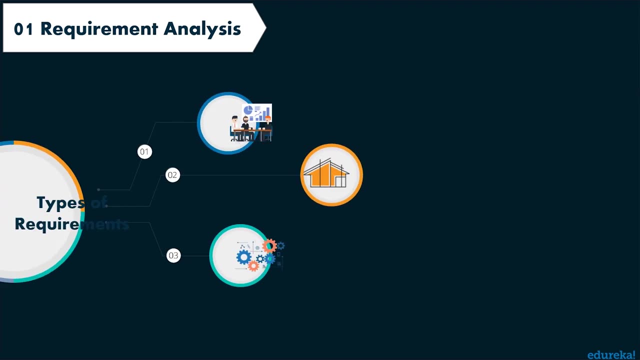 from a testing point of view, to identify the testable requirements. So the QA team may interact with various stakeholders, such as the client, business analyst, technical leads, system architects, et cetera, to understand the requirements in detail. Now let's have a look at the types of requirements. 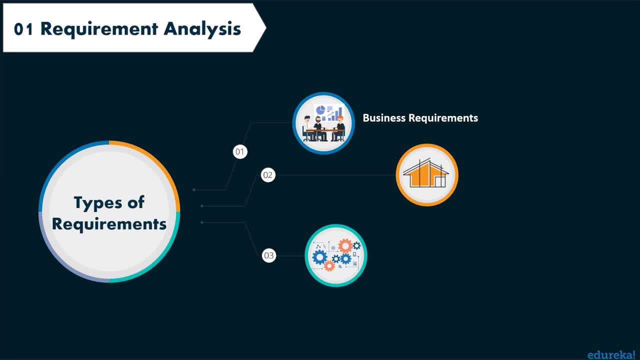 First of all we have the business requirements. Now they are high level requirements that are taken from the business case, from the projects. For example, a mobile banking service system provides banking services to Southeast Asia. Now the business requirement that is decided for India. 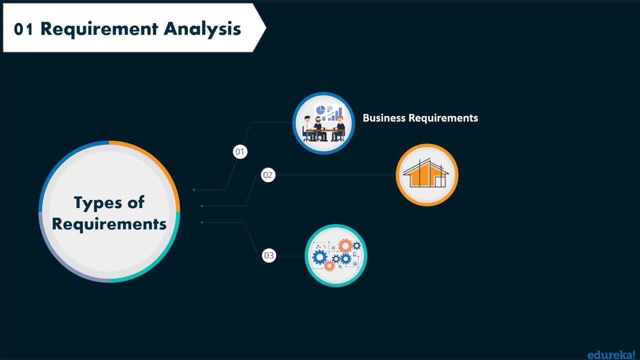 is account summary and fund transfer, while for China, account summary and bill payment is decided as a business requirement. Next up, we have the architectural and design requirements. Now, these requirements are more detailed than the business requirements. It basically determines the overall design required to implement the business requirement. 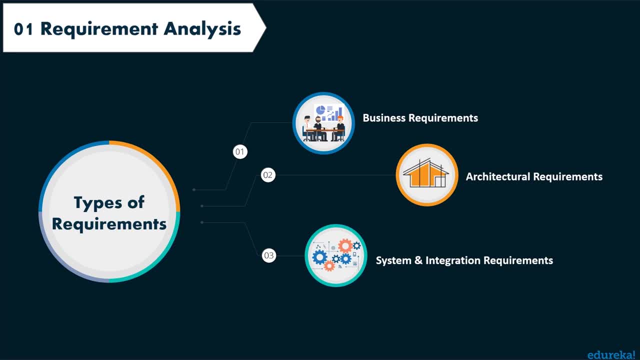 Next up is the system and integration requirements. So at the lowest level, we have system and integration requirements and it is the detailed description of each and every requirement. It can be in form of user stories, which is really describing everyday business language. The requirements are in abundant details. 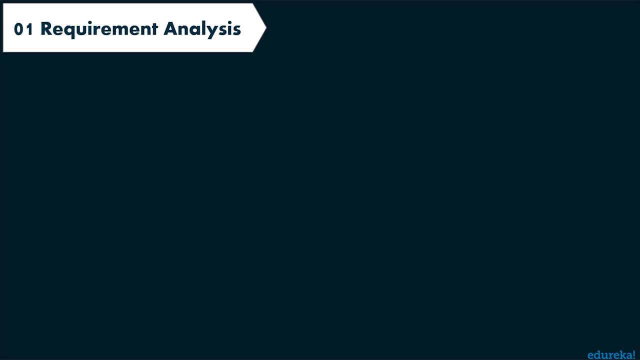 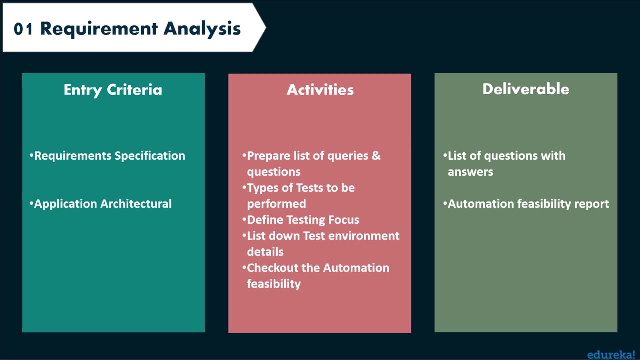 so that developers can begin coding Now. sometimes for some project you might not receive any requirements or documents to work with, but still there are other sources of requirements that you can consider for the requirement of information, so that you can base your software or test design on those requirements. 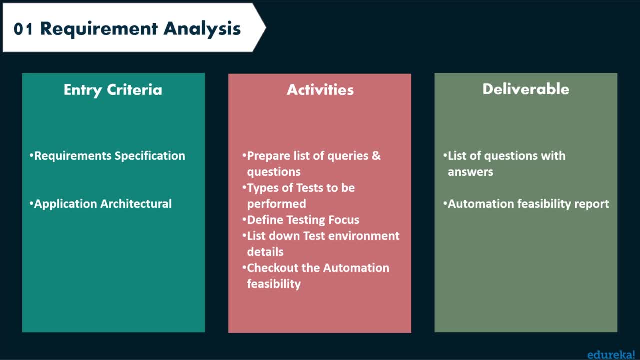 There are other sources of requirements too, such as the knowledge transfer from colleagues or employees already working on that project or talk about project to business analysts, product manager, project lead and developers. We can also analyze the domain or industry knowledge that team is trying to implement. 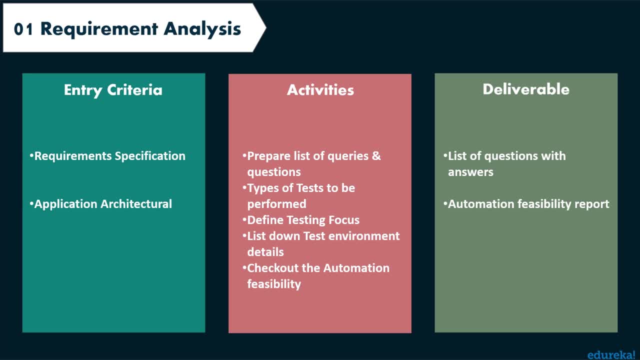 Next up, let's have a look at the entry criteria, activities and deliverables for the requirement analysis. So for entry criteria, we have requirements, specification and application architectural. Now the activities that are performed are: first, we prepare a list of queries and questions that are to be analyzed. 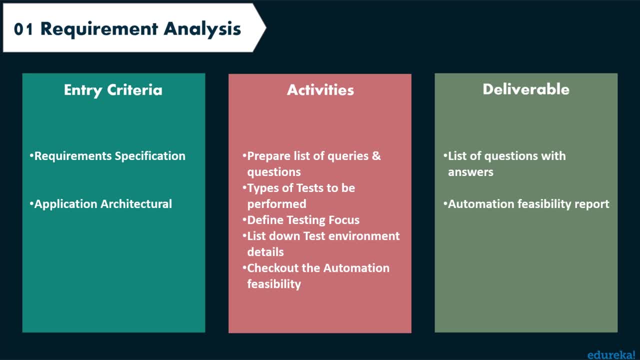 Next up, we have types of tests that are to be performed. We also define the testing focus and list down the test environment details. Finally, we also check out the automation feasibility. Now in deliverable We have all the list of questions with answers that have been asked. 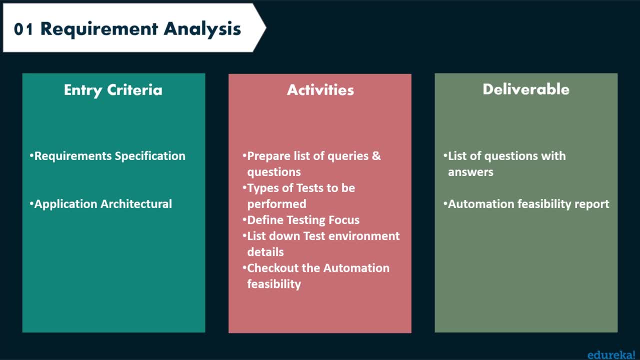 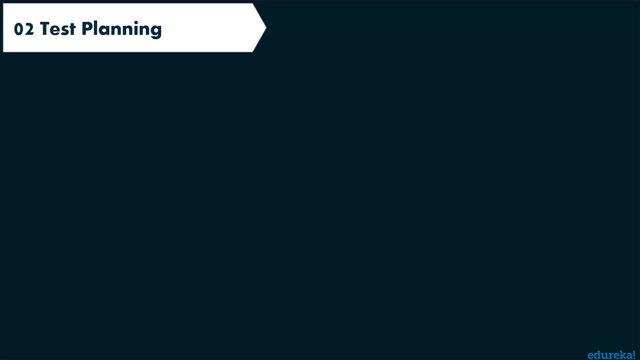 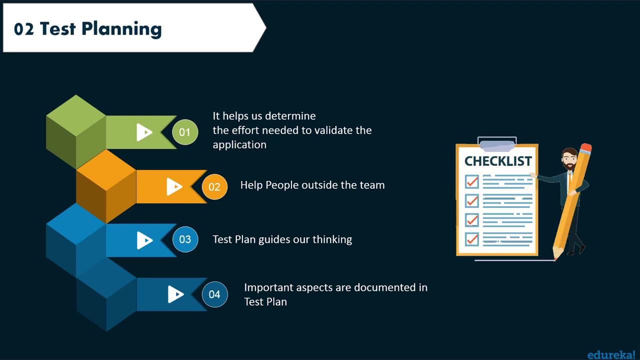 and also the automation feasibility report. So this is all about the first phase of software testing life cycle. Now let's move on and have a look at the second phase. Now, test planning is the most important phase of software testing life cycle, where all testing strategy is defined. 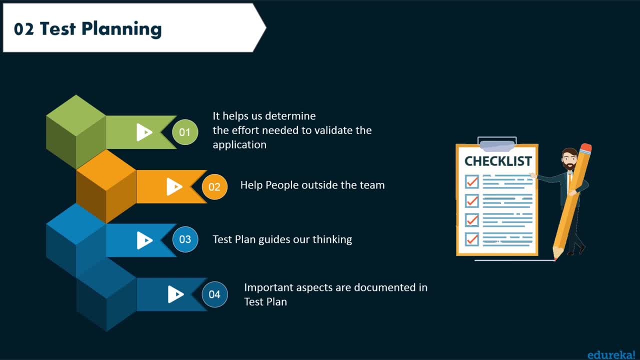 Now this phase also called as test strategy phase. in this phase, typically test manager involved to determine the effort and cost estimates for entire project. Now this phase will be kicked off Once the requirement gathering phase is completed and, based on the requirement analysis, start preparing the test plan. 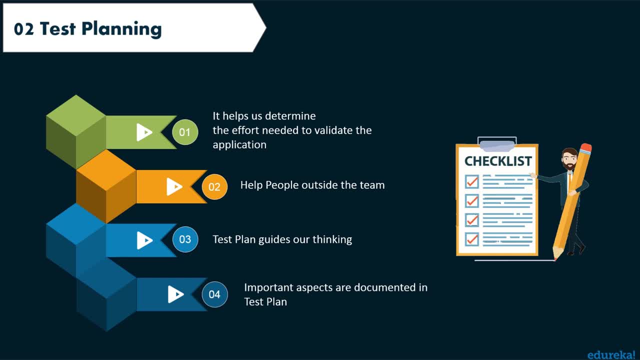 So the result of test planning phase will be test plan or test strategy and testing effort estimation documents. Once test planning phase is completed, The QA team can start with test cases development activity. Now making the test plan has multiple benefits, So test plan helps us determine the effort needed. 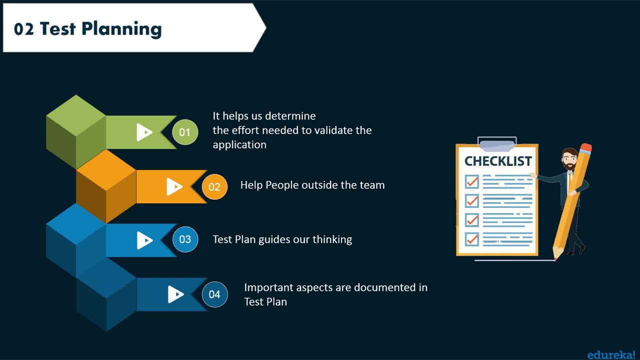 to validate the quality of the application under test. It also helps people outside the test team, such as the developers, business managers, customers, understand the details of testing. now the test plan guides are thinking it is like a rule book which needs to be followed. important aspects: 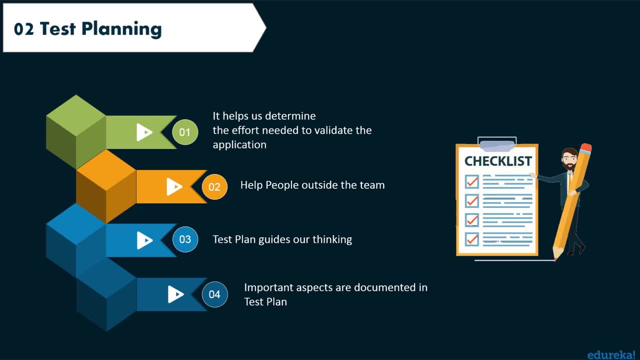 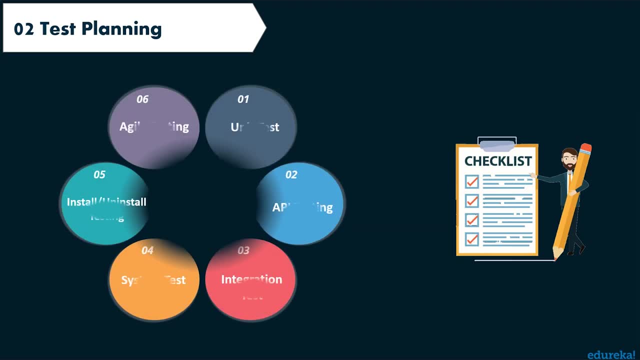 like the test estimation, test scope, test strategy, are documented in the test plan so it can be reviewed by the management team and reused for other projects. Some of the commonly used testing types are: unit test: It tests the smallest piece of verifiable software in the application. 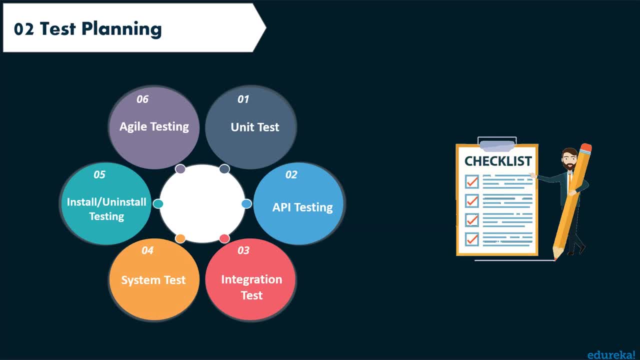 Then we have the API testing. it tests the APIs created for the application. next up, We have the integration test, So individual software modules are combined and tested as a group. next is the system test, which is conducted on a complete integrated system to evaluate the system's compliance. 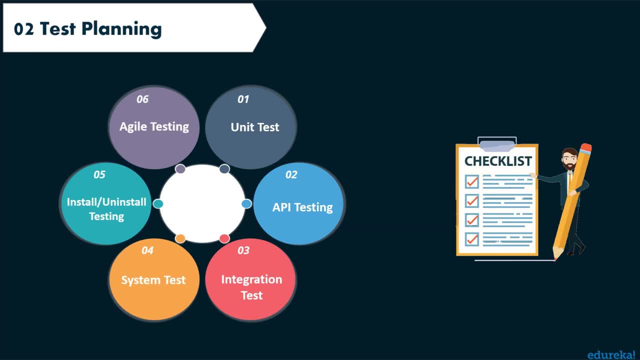 with its specified requirements. There's also install or uninstall testing, which focuses on what customers will need to do to install or uninstall and set up or remove the new software successfully. Finally, we have the agile testing. now testing the system using agile methodology is what is meant by the agile testing? 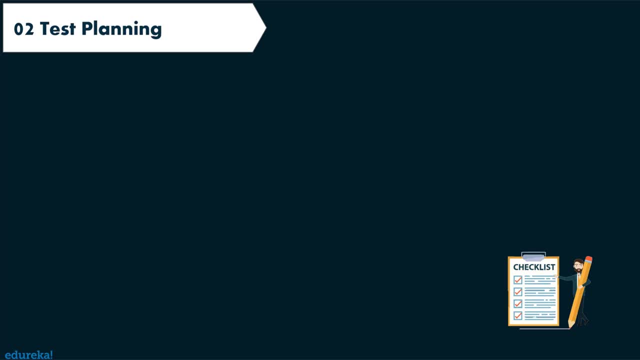 Now let's have a look at these steps involved in test planning. First We have the analyze: the product. So how can you test a product without any information about it? The answer is impossible. You must learn a product thoroughly before testing it. next up, 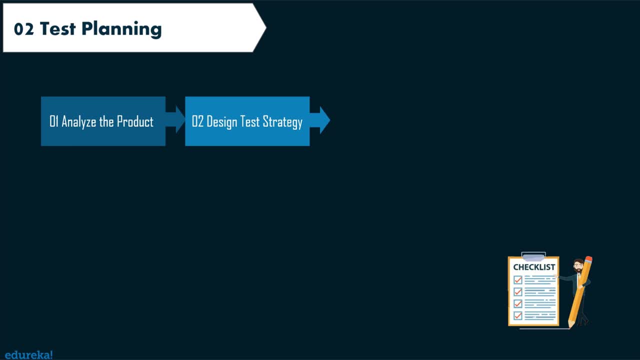 We have developed test strategy now. test strategy is a critical step in making a test plan. A test strategy document is a high-level document which is usually developed by test manager. Now this document defines the project's testing objectives and the means to achieve them. 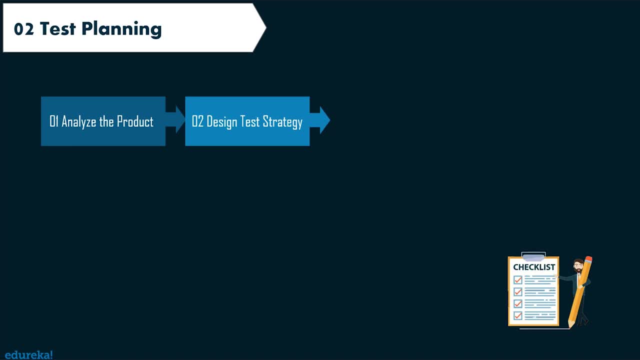 It also determines the testing effort and costs. The third step is defined: the test objective. Now the test objective is the overall goal and achievement of the test execution. The objective of the testing is finding as many software defects as possible, So ensure that the software under test is bug-free before release. 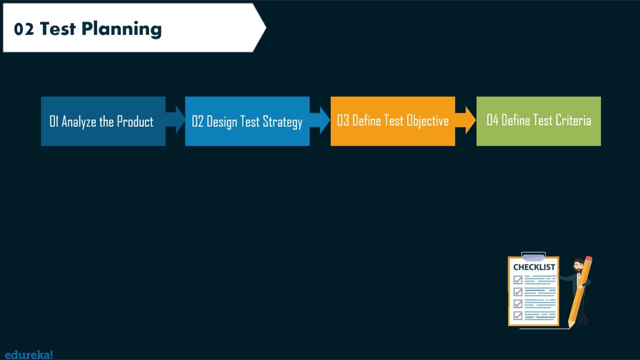 the fourth step is to define the test criteria. Now, test criteria is a standard or rule on which a test procedure or test judgments can be based, and there are two types of test criteria. The next step is the resource planning. So resource plan is a detailed summary of all types. 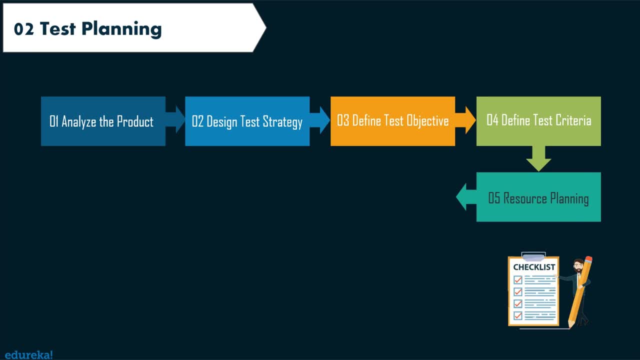 of resources required to complete project task. Now the resource could be human equipment and materials needed to complete a project. The resource planning is important factor of the test planning because it helps in determining the number of resources to be used for the project. The sixth step is the plan test environment. 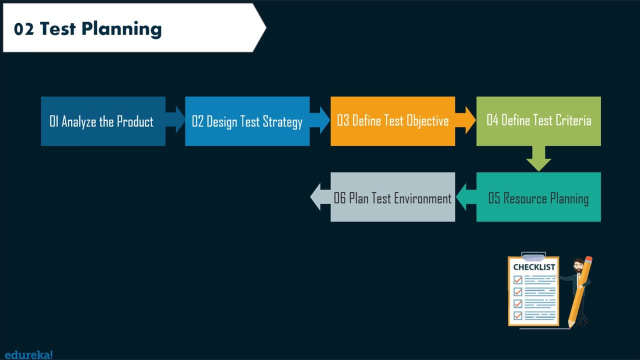 Now, what is the test environment? a testing environment is a setup of software and hardware on which the testing team is going to execute test cases. The test environment consists of real business and user environment, As well as physical environments such as server front-end running environment. 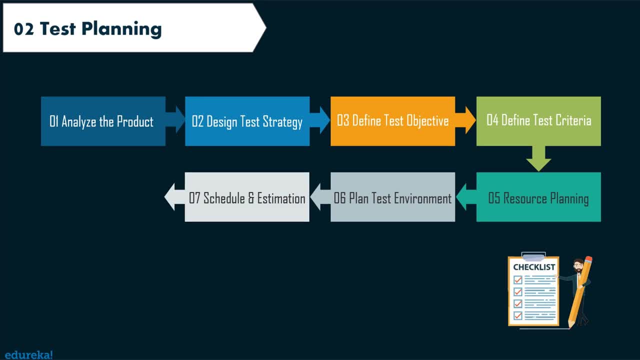 The seventh step is the schedule and estimation. now for test estimation. We use some techniques to estimate the effort to complete the project. now here you should include that estimation, as well as the schedule to the test planning. Now in the test elimination phase, suppose you break. 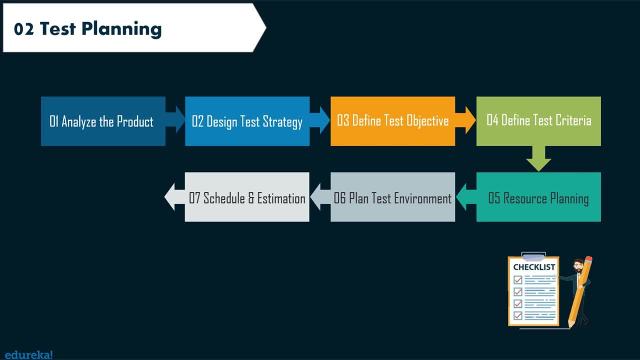 out the whole project into small tasks and add the estimation for each task. The final step is the test deliverables. Now, the test Deliverable is a list of all the documents, tools and other components that has to be developed and maintained in support of the testing effort. 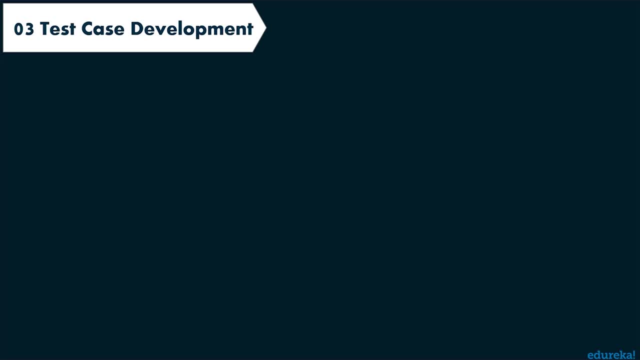 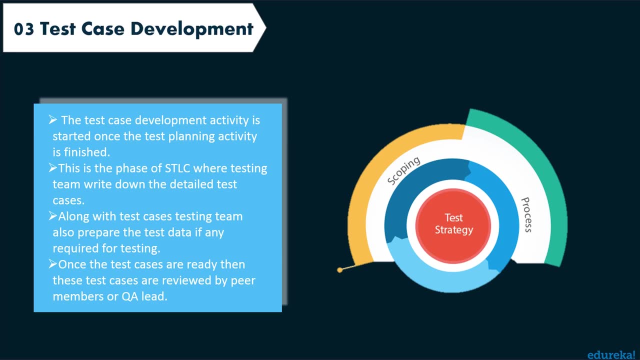 Now next up is the third phase of software testing life cycle. So the test case development begins once the test planning phase is completed. So this is the phase of software testing life cycle where testing team notes the detailed test cases. along with test cases, testing team also prepares the test data. 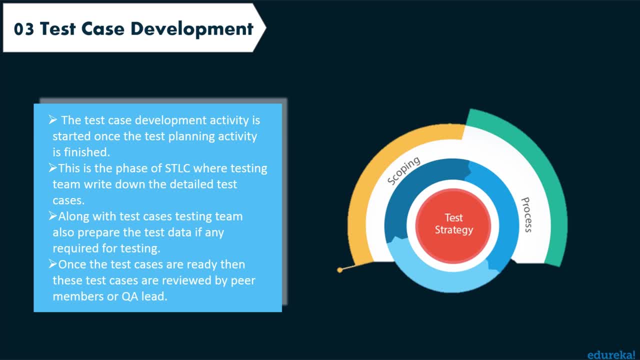 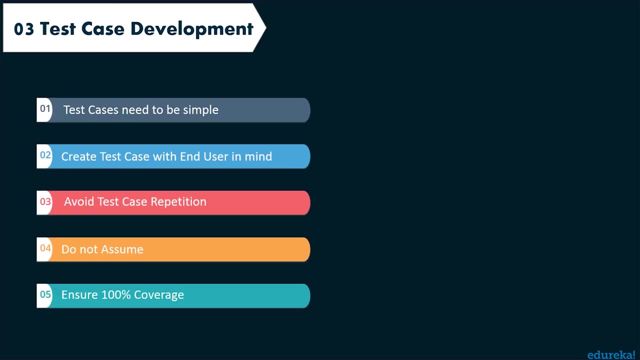 for testing. once the test cases are ready, then these test cases are reviewed by peer members or QA lead. So a good test case is the one which is effective at finding defects and also covers most of these scenarios on the system under test. So here is a step-by-step guide. 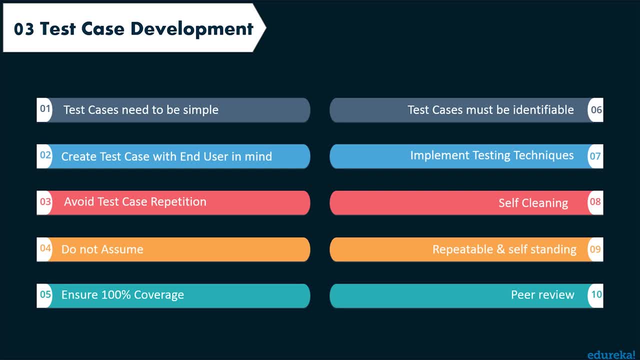 on how to develop a good test case. First of all, the test cases need to be simple and transparent. So first we have to create test cases that are as simple as possible. They must be clear and concise, as the author of the test case may not execute them. 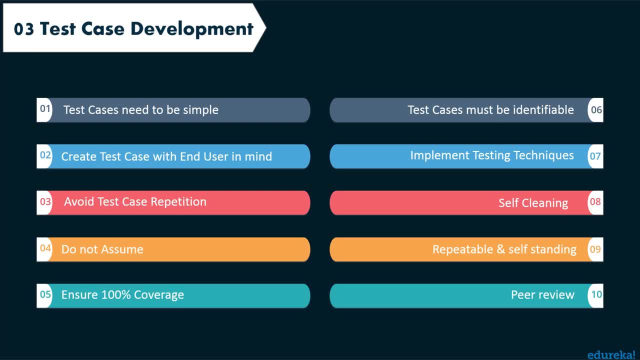 So we have to use assertive language like: go to the home page, enter data, click on this and so on. So this makes the understanding, the test steps easy and test execution faster. next, We should create test case with end user in mind. So the ultimate goal of any software project is: 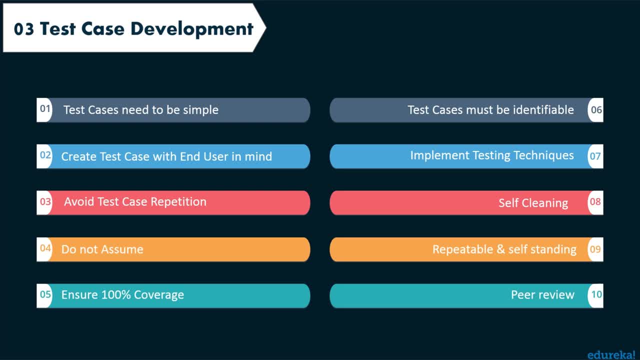 to create test cases that meet customer requirements and is easy to use and operate. So a tester must create test cases Keeping in mind the end user perspective. The next step is to avoid the test case repetition. Now do not repeat test cases If a test case is needed for executing some other test case. 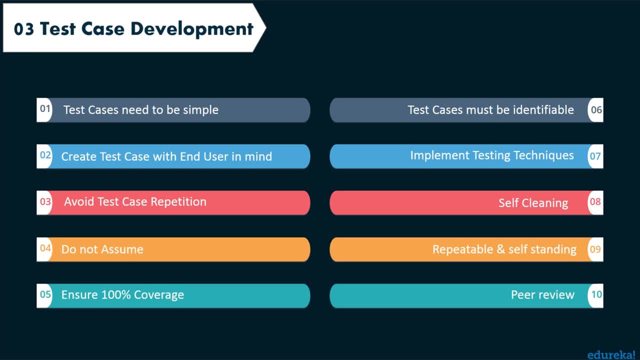 on the test case by its test case ID in the precondition column. do not assume so. do not assume the functionality and features of your software application while preparing test case. stick to the specification documents. also ensure hundred percent coverage. Make sure you write test cases to check all software requirements mentioned. 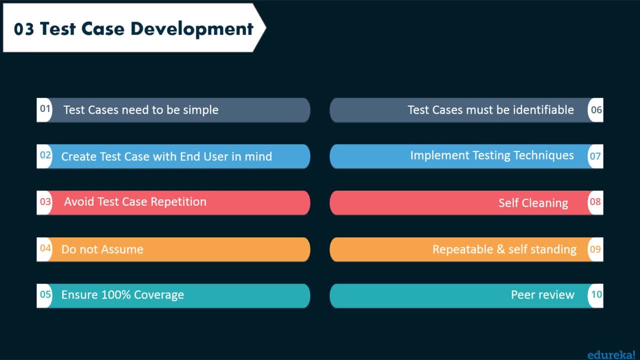 in the specification document. So use traceability Matrix to ensure no functions or conditions is left untested. next up, The test cases must be identifiable. now name the test case ID such that they are identified easily while tracking defects or identifying a software requirement at a later stage. 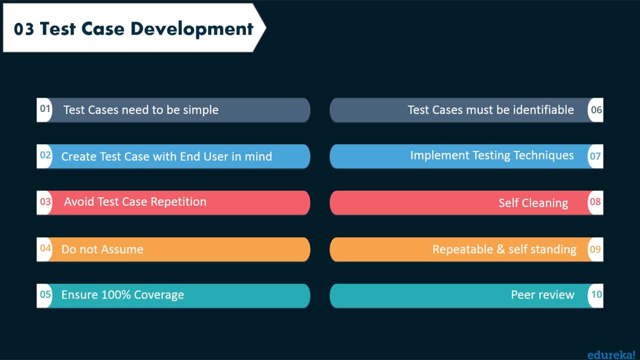 The next point is implement testing techniques. Now it's not possible to check every possible condition in your software application, So software testing techniques help you select a few test cases with the maximum possibility of finding a defect. for that We have the boundary value analysis, as the name suggests. 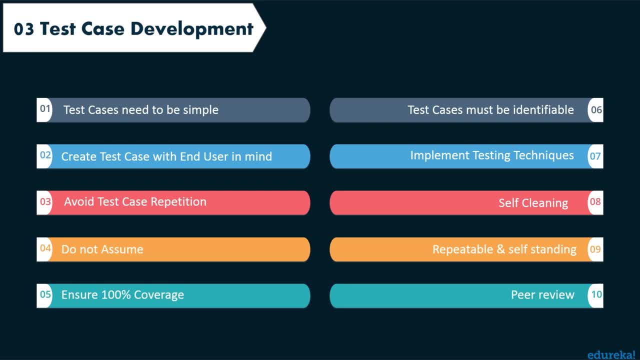 It's the technique that defines the testing of boundaries for a specified range of values. Also, we have the equivalence partition. now this technique partitions the range into equal parts or groups that tend to have the same behavior. Next is the self-cleaning. So the test case you create must return the test environment. 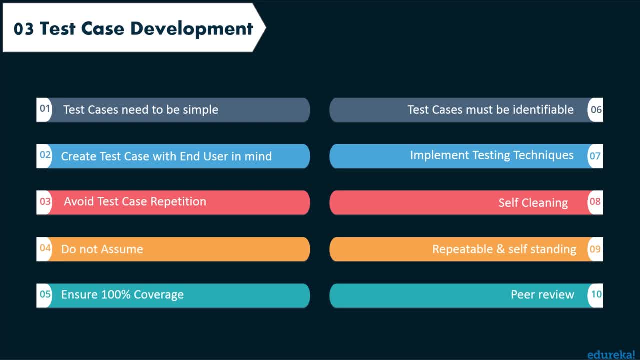 to the pre-test state and should not render the test environment unusable. Now, this is especially true for configuration testing. Next point is the repeatable and self-standing, So the test case should generate the same results every time, no matter who tests it. and the final point is the peer review. 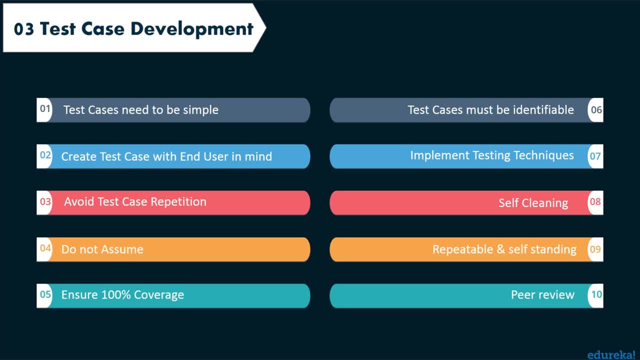 So, after creating test cases, get them reviewed by your colleagues. your peers can uncover defects in your test case design which you may easily miss. So these were some of the guidelines in order to build a good test case development. Now moving on next up. 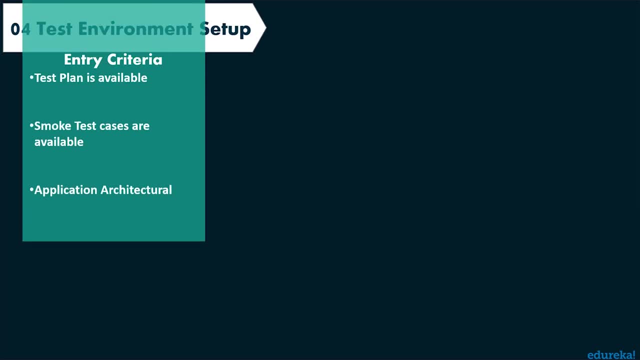 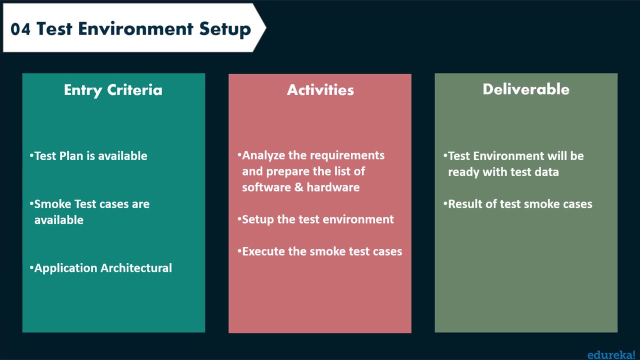 We will see the test environment setup phase of software testing lifecycle now. setting up the test environment is the vital part of the software testing lifecycle. a testing environment is a setup of software and hardware for the testing teams to execute test cases. It supports test execution with hardware software. 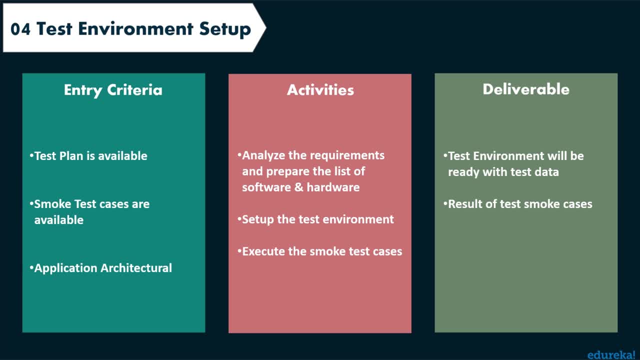 and Network configured. So let's have a look at the entry criteria. So first we have the test plan available, Then we have smoke test cases and finally the application architectural. now in activities. First we have to analyze the requirements and prepare the list of software. 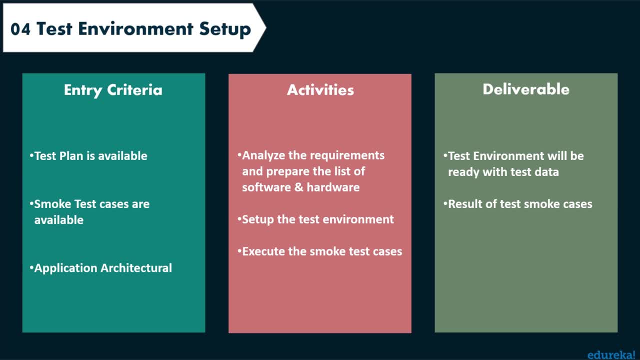 and hardware required to set up test environment. Next, we have set up the test environment And finally, once the test environment is set up, Execute the smoke test cases to check the readiness of the test environment. now, in the deliverable section, the test environment will be ready. 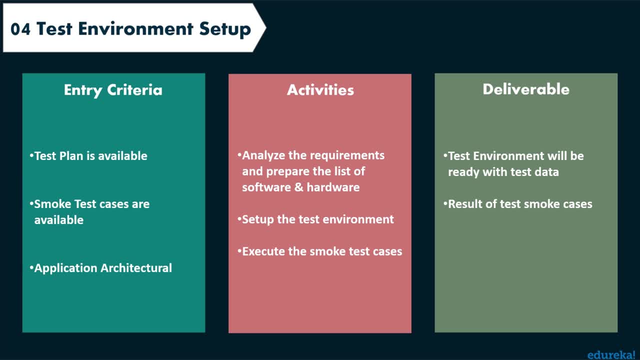 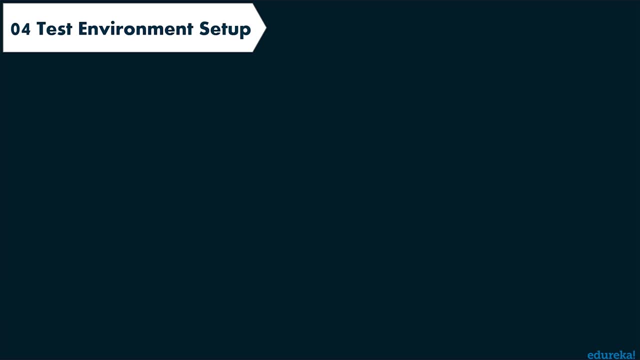 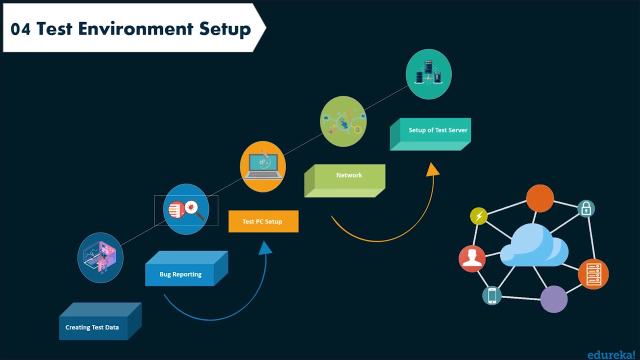 with test data. Also, the result of the smoke test cases are delivered here Now. the test environment also involves setting up of distinct areas like setup of test server. So every test may not be executed on a local machine. It may need establishing a test server. 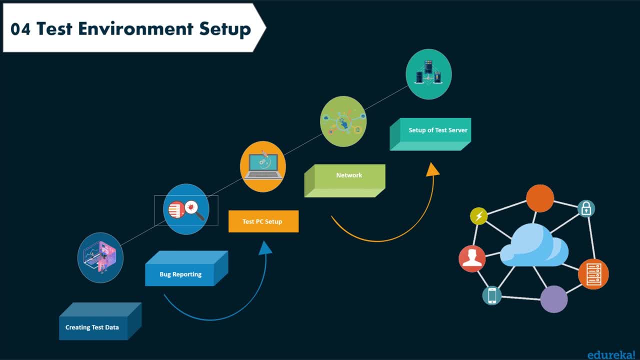 which can support application applications. next up is the network, So we need to set up the network as per requirements. We also have the test PC setup, So we need to set up different browsers for different testers. next up, We have the bug reporting. 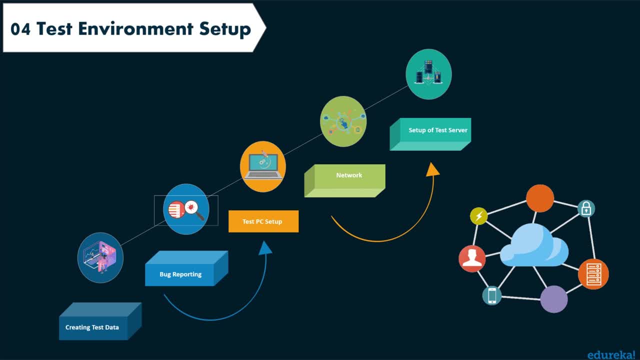 So the bug reporting tools should be provided to the testers. Finally, we have the creating testing data for the test environment. Now many companies use a separate test environment to test the software product, So the common approach used is to copy production data to test now. 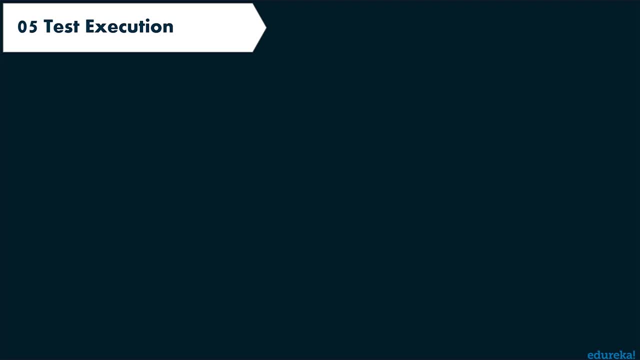 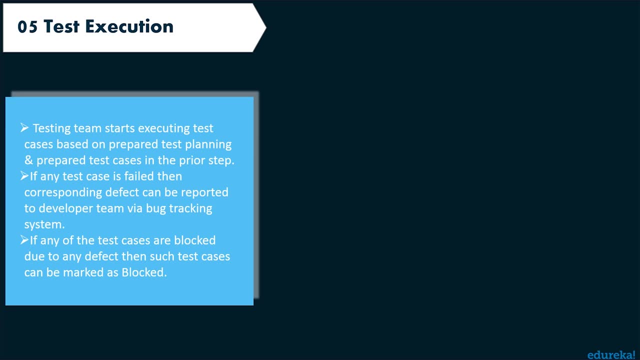 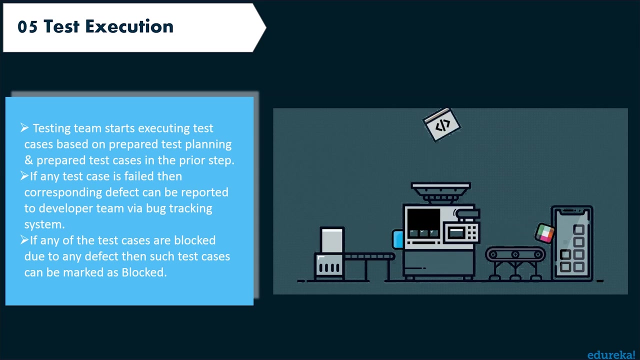 let's move on to the fifth phase of software testing life cycle. So the next phase is test execution. Now, test execution is the process of executing the code and comparing the expected and actual results. So when test execution begins, the test analyst start executing the test scripts based on test strategy allowed in the project. 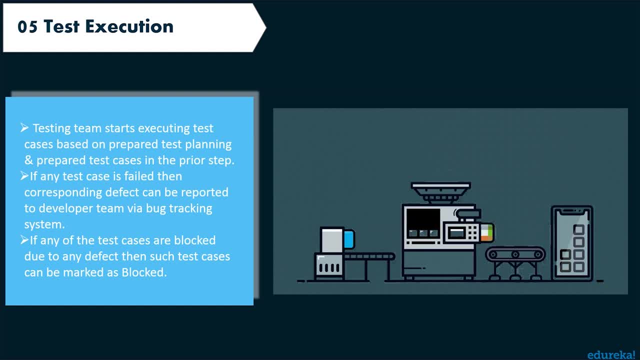 So the testing team starts executing test cases based on prepared test Planning and prepared test cases in the prior step. if any test cases fails, then corresponding defect can be reported to developer team via the bug tracking system. Also, if any of the test cases are blocked due to any defect, 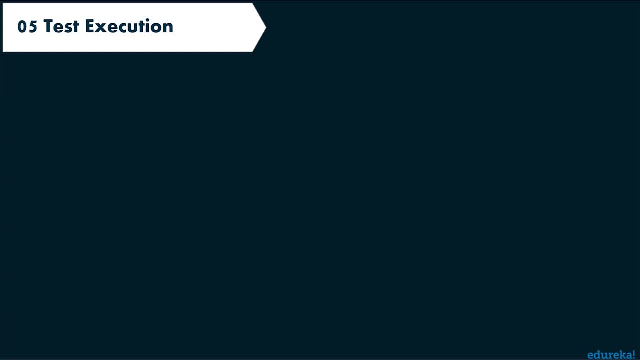 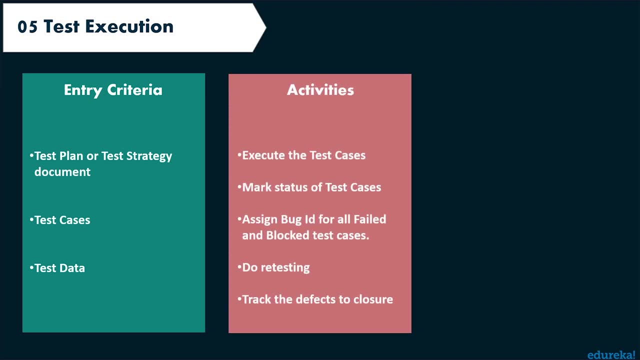 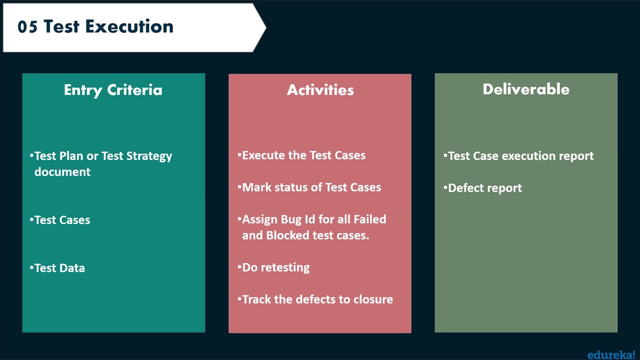 then such test cases can be marked as blocked. Now let's have a look at the entry criteria of test execution. So we have the test plan or test strategy document. Then we would need the test cases and also the test Data and activities performed. here are. so first we have 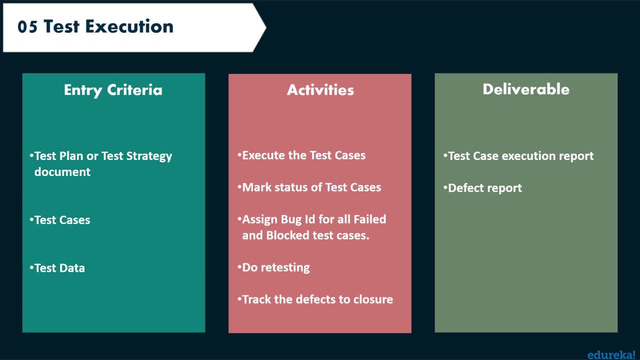 to execute the test cases and then we have to mark status of test cases like passed, failed, blocked, not run, Etc. Then we have to assign the bug ID for all failed and blocked test cases. We also have to do the retesting once the defects are fixed. 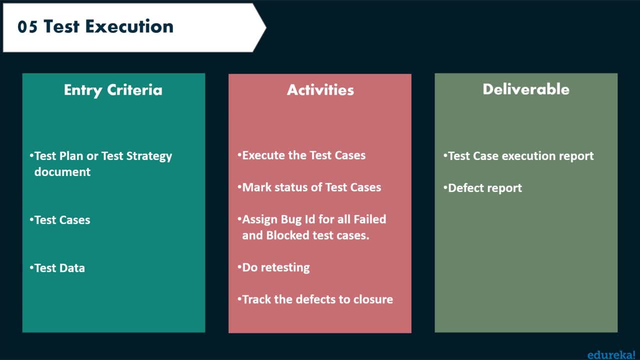 and finally track the defects to closure. in the deliverable section We will have the test case execution report and also the defect Report of our test. Now, Finally, we are here at the final phase of software testing life cycle. The final phase is the test cycle closure. 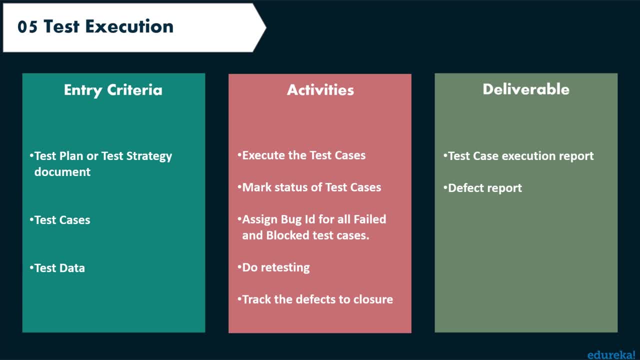 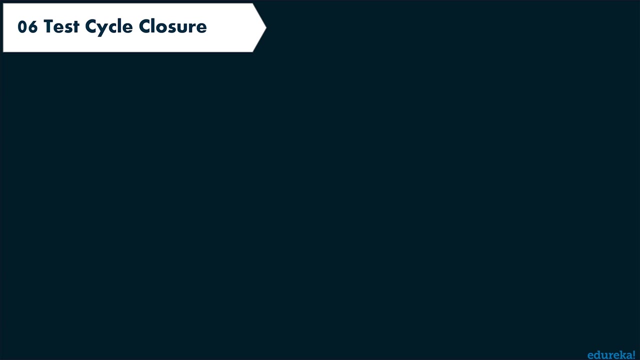 Now this involves calling out the testing team member meeting and evaluating cycle completion criteria based on test coverage, quality, cost, time, critical business objectives and software. So a test closure report by the test lead is published after accomplishing the exit criteria And finishing the testing phase. 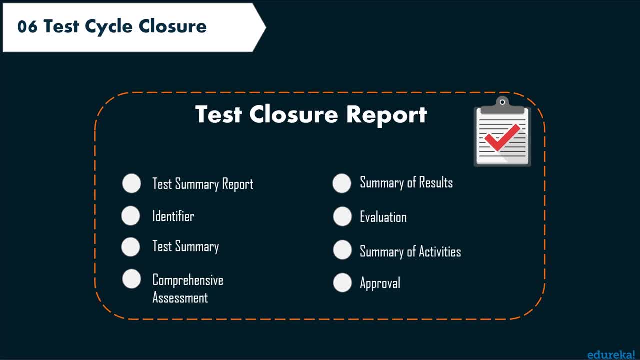 and it also follows a standard format, such as we have the test summary report, We have an identifier, a test summary, variances, comprehensive assessment, summary of results, evaluation, summary of activities and also the approval. So this is the test closure report that we receive at the end of our test cycle closure. 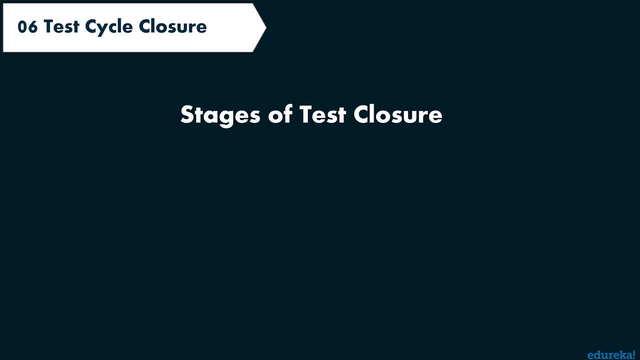 Now let's have a look at all the stages of test closure. now the process of test closure is implemented with the assistance of six important stages, which helps the team check and validate various components of the software before it is released for the end users. 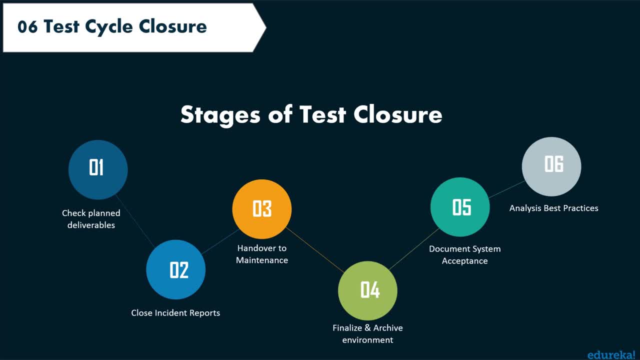 Now these stages involves continuous engagement of the testers, as well as the team leads or manager, where they take measures to ensure the quality and effectiveness of the software. Hence, the six important stages of test closure are: check plant deliverables. Now the plant deliverables that will be given to the stakeholder of the project are checked. 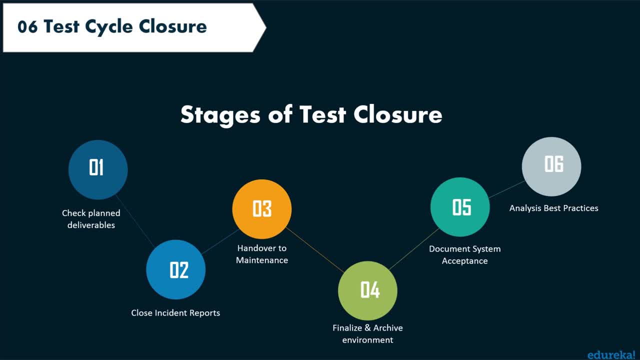 and analyzed by the team. These mainly include test case documents, test plan, test strategy, test scripts, test data traceability matrix and test results and reports like test closure report. Moreover, the team here ensures that all of these plant deliverables are delivered to these stakeholders. 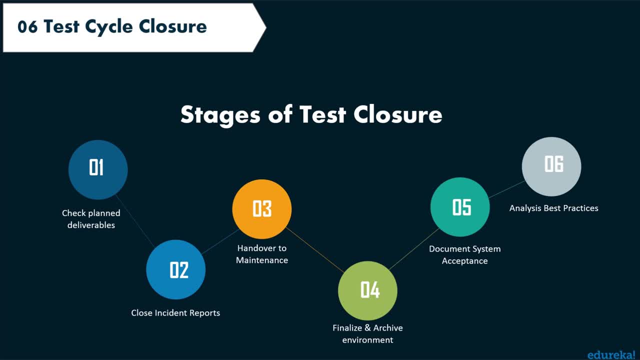 Next step is the close incident reports. Now, incidents are the variations and deviations observed by the team in system behavior during the process of testing. These are logged as a report in the earlier stages and closed during this stage of process. here The team checks that the plant deliverables are delivered. 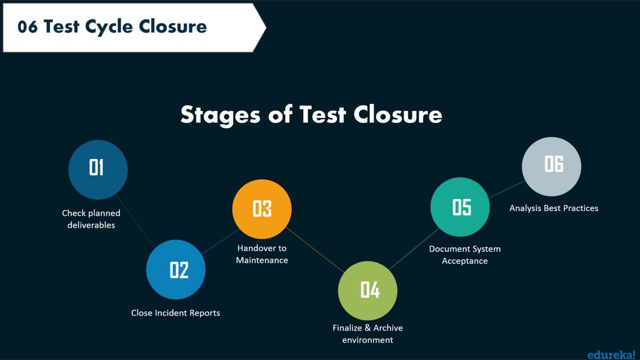 and validates that all the incidents are resolved before the culmination of the process. next up, We have the handover to maintenance. now, after resolving incidents and closing the incident report, The testwares are then handed over to the maintenance team, who provide their adept support to the software during its release. 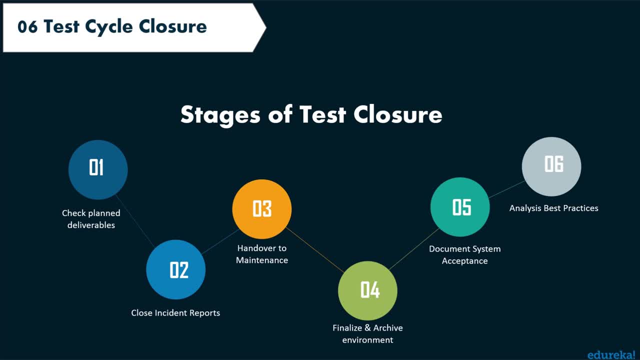 and client-side implementation. The next step is finalize and archive the testware or environment. Now, during this stage of test closure, involves finalizing and archiving of the testware and software, like test scripts, test environment, test infrastructure, etc. for later use. The fifth step is the document. 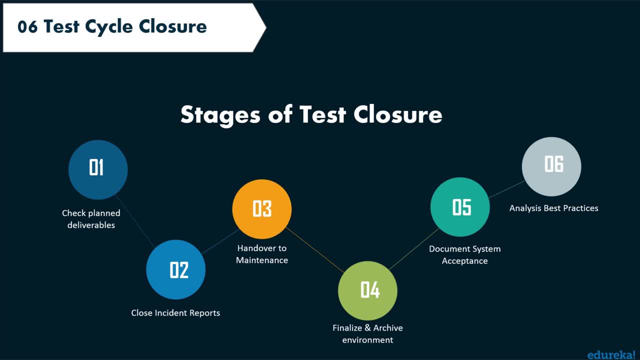 system acceptance. now, here, every aspect of the developed software and application, along with its supporting data and information, is accepted by the customer representatives before the implementation of the software system. Now this involves system verification and validation according to the strategy outlined and defined in the validation section. 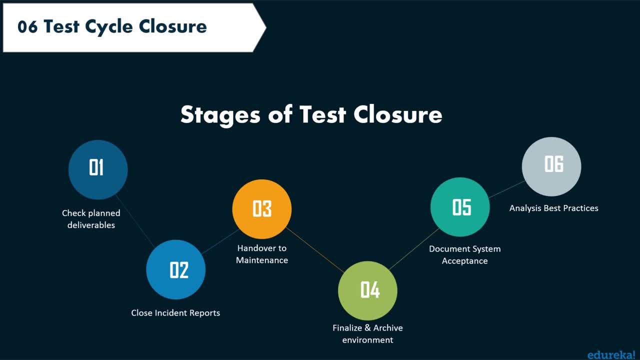 The final step is analyzing the best practices. Now this is the last stage of test closure, wherein the learned lessons are analyzed for future references. This helps us determine the various changes that might be required for similar projects and their future release. Moreover, this information is gathered.